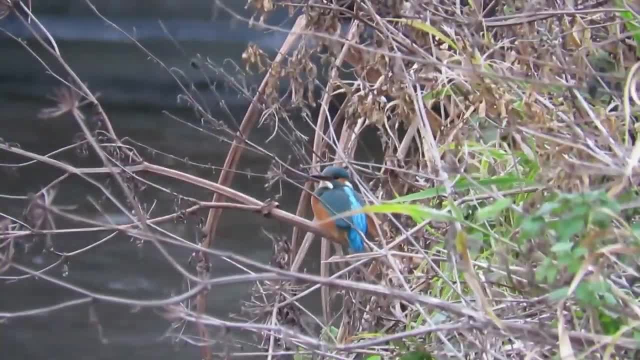 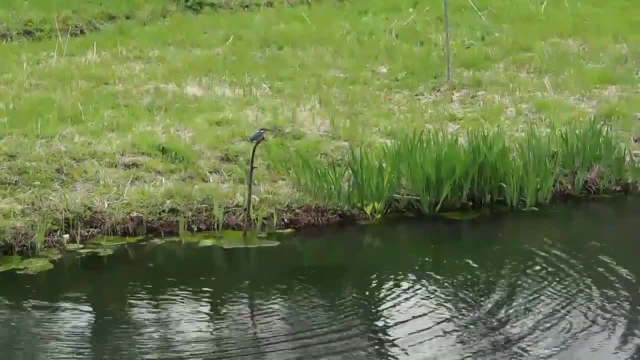 in length. Kingfishers most often hunt from a perch, although some species are capable of hovering while they hunt and can fly over deep water to catch food. Those that dive often have a membrane that closes over their eye when they enter the water, so they have to catch their 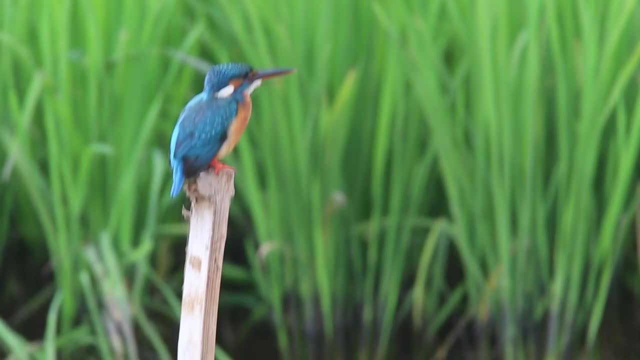 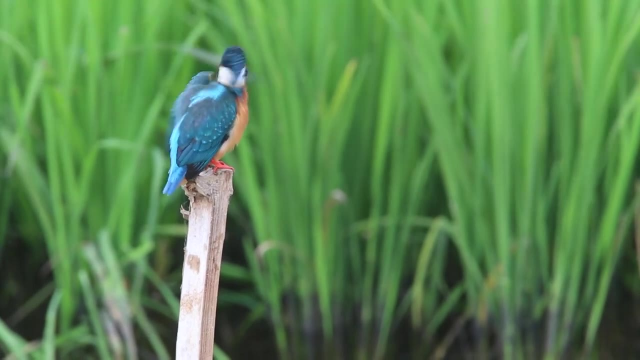 quarry by feeling and not sight. Once a meal is captured, the kingfisher returns to its perch and jabs the prey with its beak. Kingfishers are also known for their sharp, sharp, sharp, sharp beak, often smacking it against the perch to make it easier to swallow. 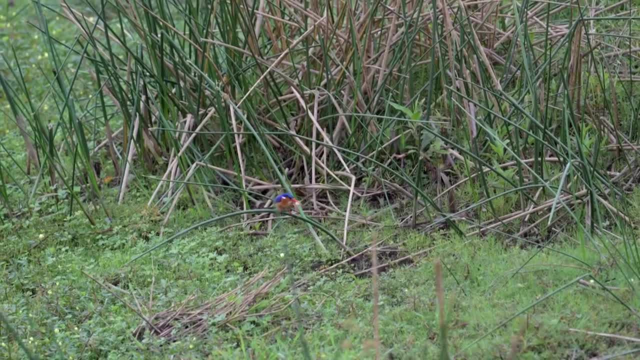 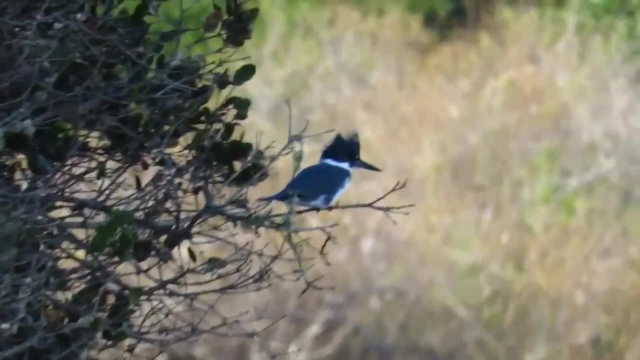 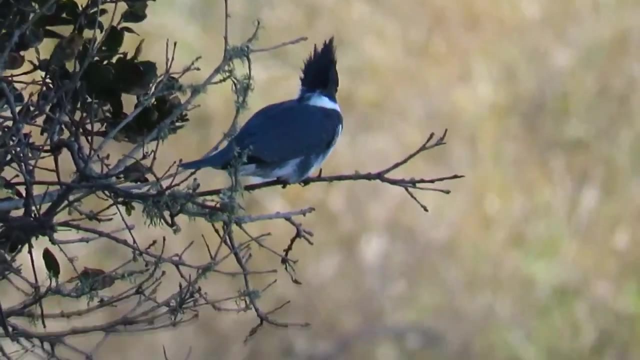 Kingfishers have long beaks, short necks and wings and fused toes. They're generally capable enough flyers that adults are rarely predated. However, nest invaders include all kinds of animals such as chimps, raccoons, minks, dingoes, monitor, lizards and more. 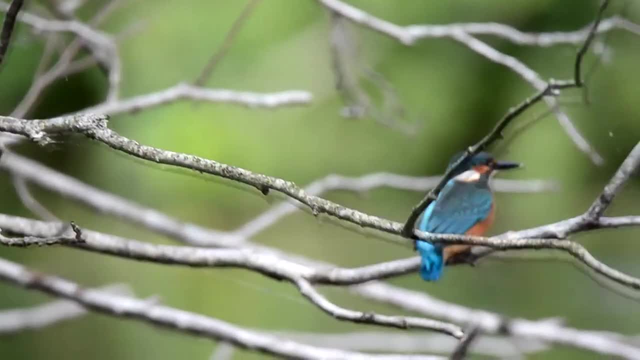 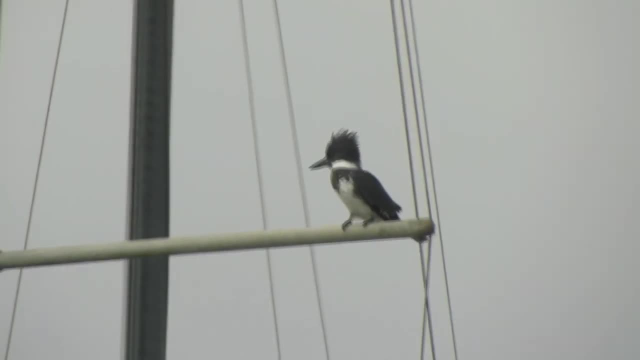 Kingfishers are recorded reaching 15 years of age, although the lifespan of many species is unreported. Kingfishers are also known for their sharp, sharp, sharp, sharp, sharp, sharp beak. These birds start life as an egg. A female lays about two to eight eggs in a nest. 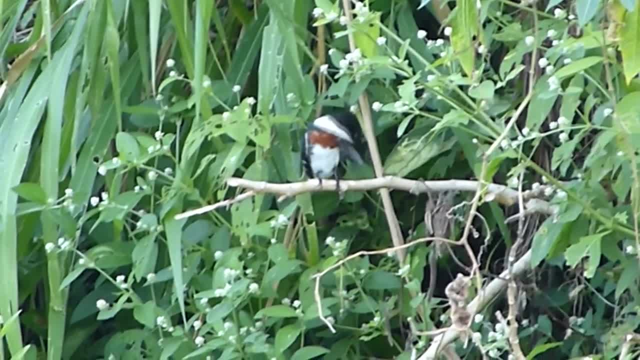 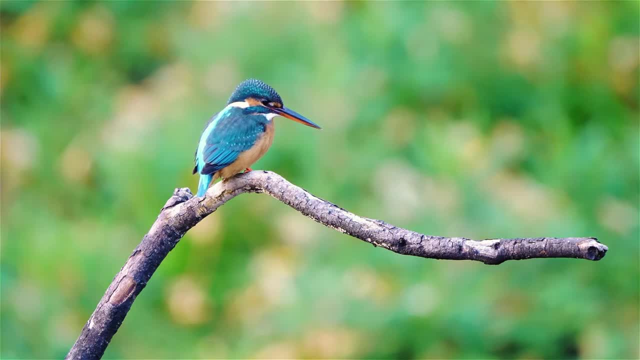 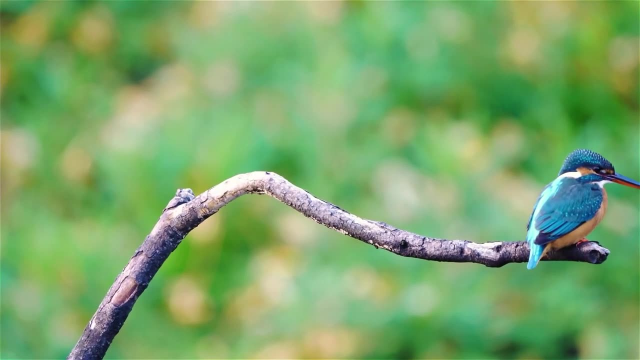 constructed by both parents. Kingfishers commonly utilize earthen hillsides which they excavate to form nesting chambers. If this isn't available, they'll also use the burrows of other animals, including termites, or take over the excavated holes of other animals, such as woodpeckers. 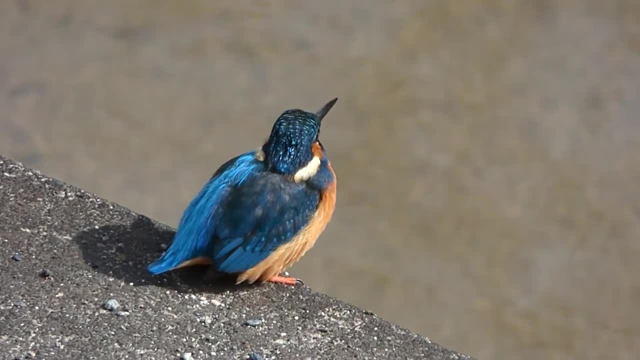 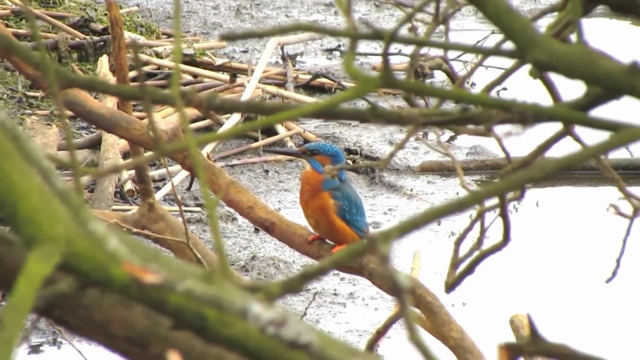 Both parents incubate the eggs and they take about a month to hatch. The chicks stay in the nest for another month until they hatch, and then they hatch again. The chicks stay in the nest for another month before emerging to learn how to fly and hunt In diving species. 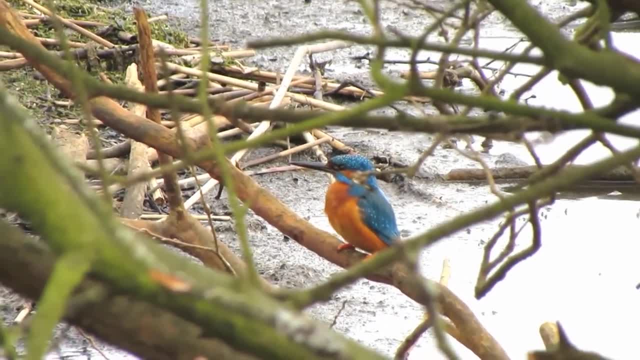 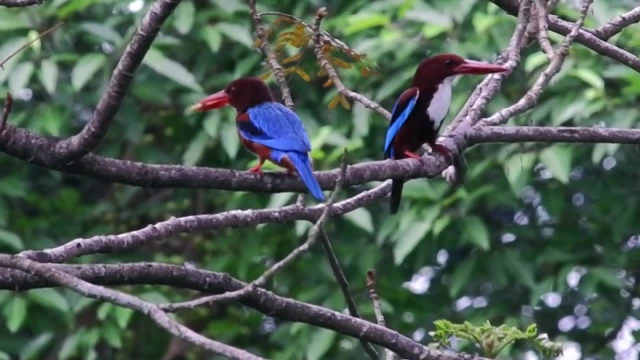 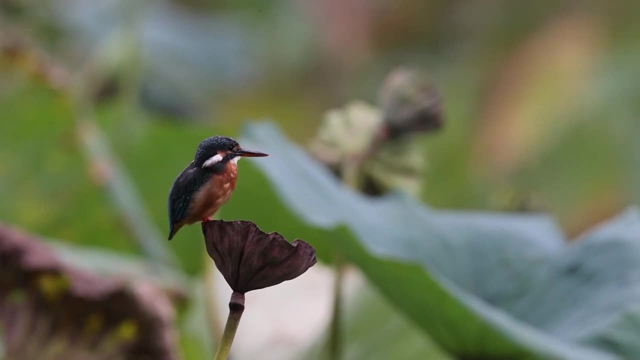 the parents leave out nearly dead fish for the babies to practice. Many kingfishers live in monogamous pairs, which defend their territory from any intruders, including humans. There are some species that have nesting helpers, either their own, young from previous years or even unrelated individuals. 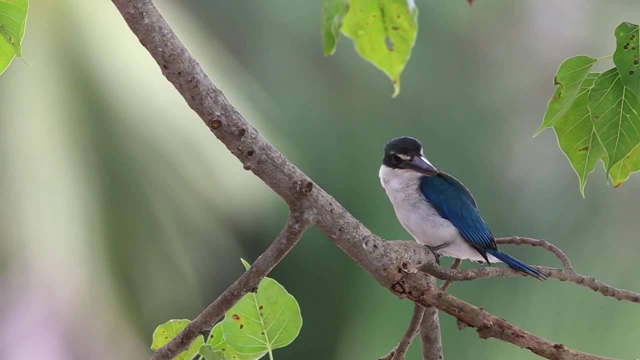 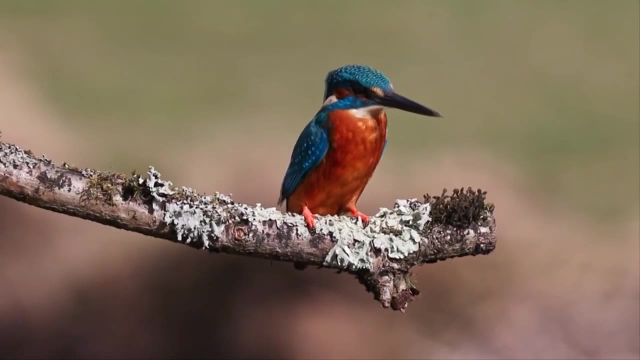 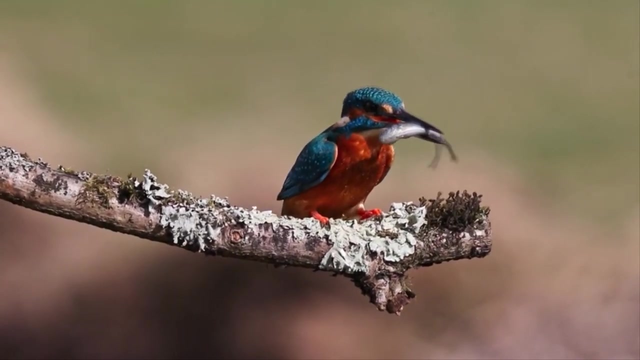 These helpers are non-breeding and ensure the chicks survive to independence. In situations where this occurs, the chicks are far more likely to live. Kingfishers may also infrequently form loose colonies of multiple breeding pairs. This occurs when nesting sites are few and far between, so the birds must cooperate to.